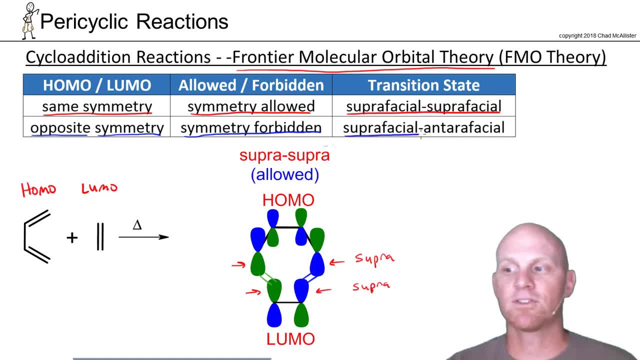 product and stuff, But the result is from what we call a suprafacial and terafacial interaction, a suprafacial and terafacial transition state, And we'll see a little more of what this means on the next slide. Okay, so the reaction we have sitting in front of us is no longer a. 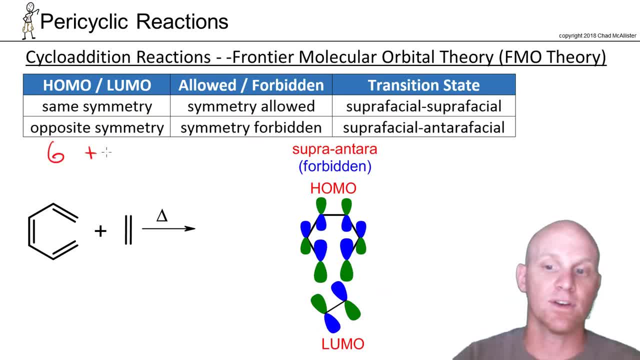 Diels-Alder reaction. It's a superfacial and terafacial transition state And we'll see a 4 plus 2 cycloaddition. It's now a 6 plus 2 cycloaddition And things are going to be a. 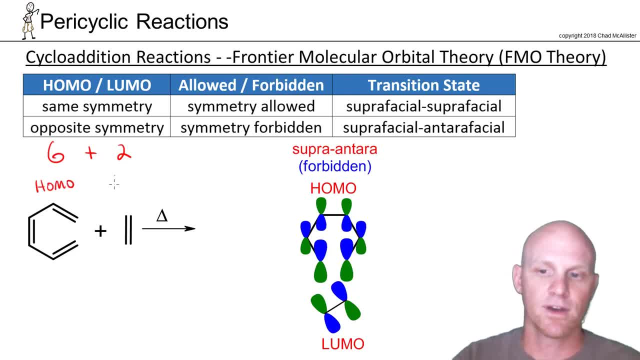 little bit different. So we want the HOMO of the conjugated system interacting with the LUMO. In this case it's not really a dienophile anymore. It might be a trienophile in this case or something. But the other pi system here- And if you recall his LUMO is going to be pi 2 or psi 2- 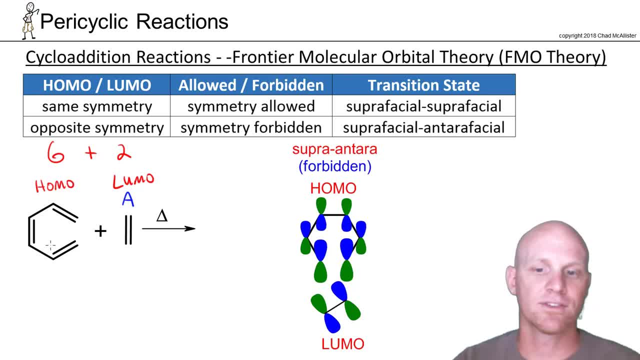 and be antisymmetric, Whereas this guy, his HOMO, with 6 pi electrons, the first three molecular orbitals are full, And so that 3 pi electrons are full, And so that 3 pi electrons are full, And so that third one, psi 3, is going to be the HOMO. So, in this case being psi 3, that's going to be. 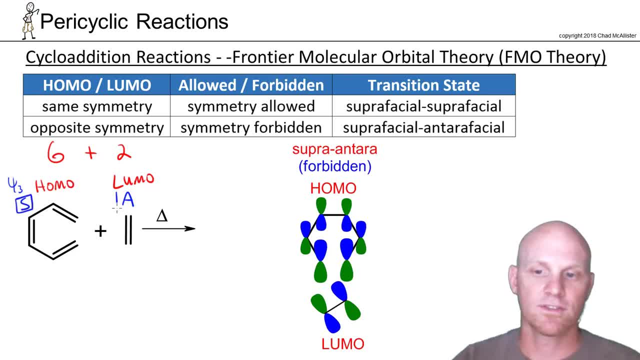 symmetric And we see we have a problem- One's symmetric, one's antisymmetric- If we try to line them up. so if I try to interact, the top face here, one side. so far, so good. The problem is is that's not going to work here. These don't match, They're not in phase And I'm not going. 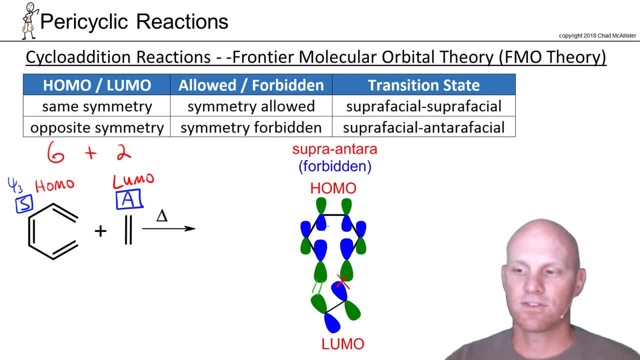 to easily form a bond there, And so what has to happen is this arrangement has to kink. One of the two reactants has to kink, And that's why I've kind of turned this one sideways, And so what we're going to try and do here is actually have this interact here instead. 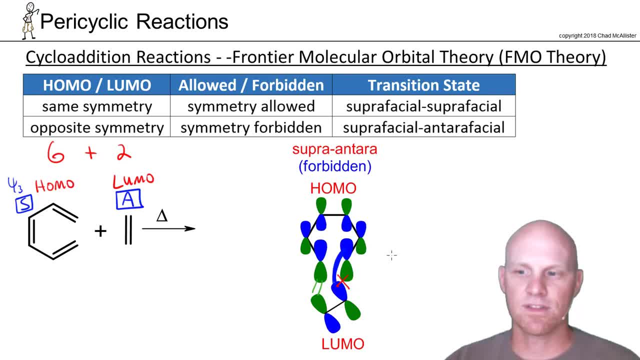 And so we end up having, you know, a little bit different interaction than we think we have. So in this case, one of the reactants is interacting with the top lobes on both sides, and that's suprafacial, But the other one is interacting with the bottom lobe on one side, but the top 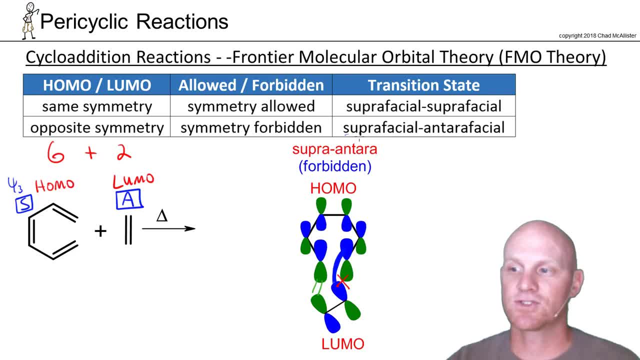 lobe on the other side and that's antarafacial And that's with this idea of suprafacial and terafacial comes from. So, and this is absolutely forbidden, So, and just like when you're absolutely forbidden in high school to stay out past 11 o'clock or something like that. 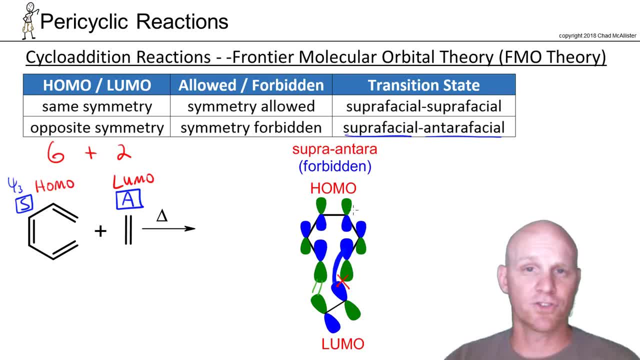 well, does that mean it's never going to happen? No, it just means your parents forbade it and you're going to get in trouble. but it's still going to happen. Same thing here: When we say something's forbidden in this context, it doesn't mean that that reaction can't. 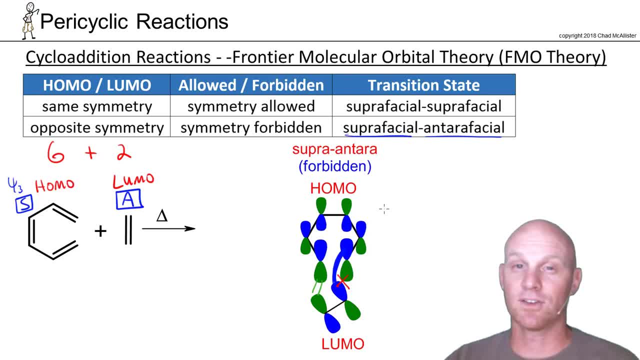 happen necessarily. It just means it's not as likely and you're not going to get as good a yield of it in any way, shape or form. So just because this is forbidden doesn't mean it's not going to happen. So in this case we could form a new sigma bond right here and a new one right here. 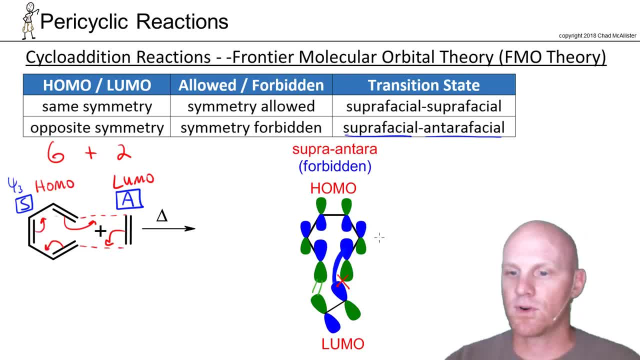 and kind of go around the horn And in this case we're going to form an eight-membered ring and we'll have pi bonds here and then we'll have a couple of new sigma bonds, both here and here. But that's our product, So and it's forbidden product. And again, that doesn't mean it doesn't. 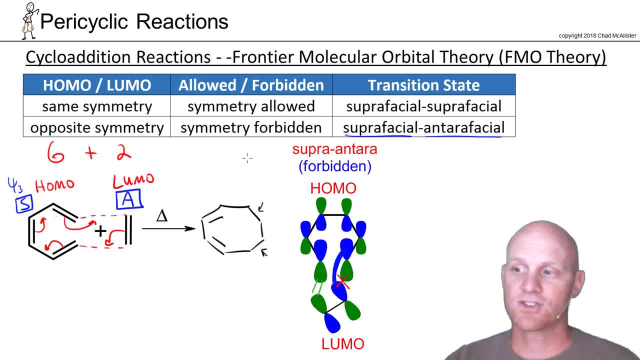 form, but it probably means it's not going to happen. So and this is forbidden. So, and this is forbidden because we're not going to get a whole lot of it, So, but it would have a superfacial and terafacial transition state. It is symmetry forbidden because, again, your HOMO for 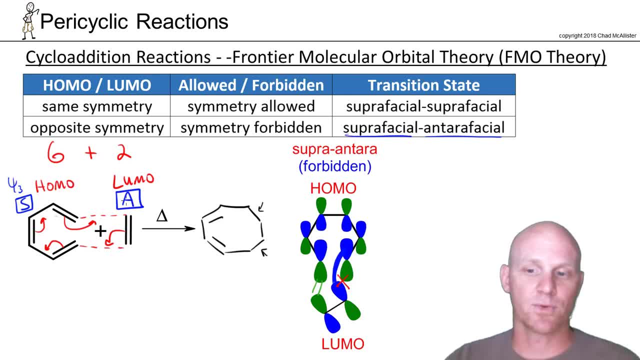 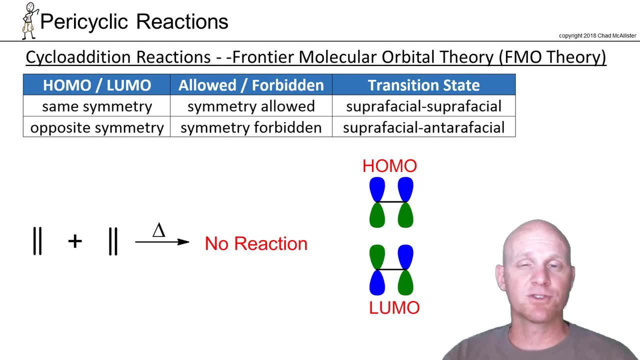 Psi 3 was symmetric and your LUMO Psi 2 for the other reactant was anti-symmetric. So in this next example we want to look at a symmetry forbidden reaction that actually is also geometrically forbidden and doesn't actually occur. In this case we've got two ethylenes. 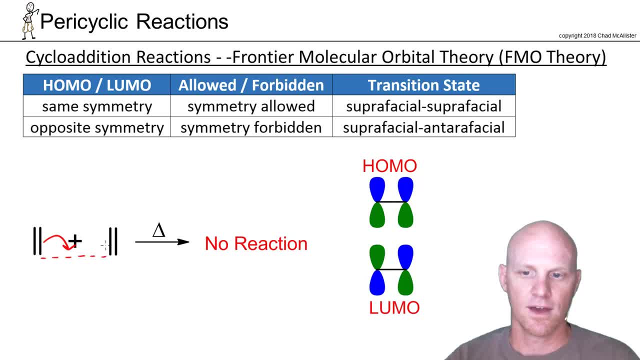 and the question is: can we do the cyclic motion of electrons And form a four-membered ring? So if we kind of envision that it looks like, well, sure, it looks like the arrows look good, Shouldn't I just get you know cyclobutane? It looks beautiful. 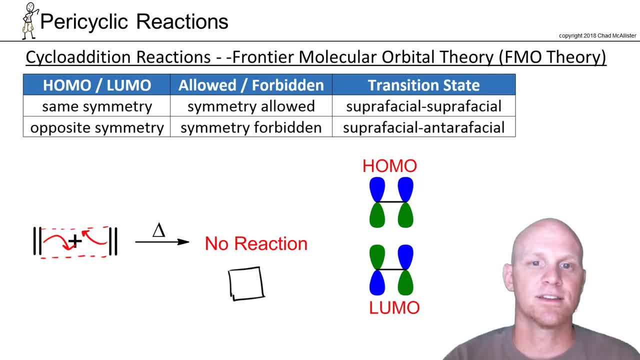 Well, it turns out, no, and it turns out you get no reaction. And again, this idea of you know, conservation of symmetry is kind of how we explain why no reaction occurs. So if we look here, so we want to use the HOMO of one of the reactants interacting with the LUMO of the other one. Well, 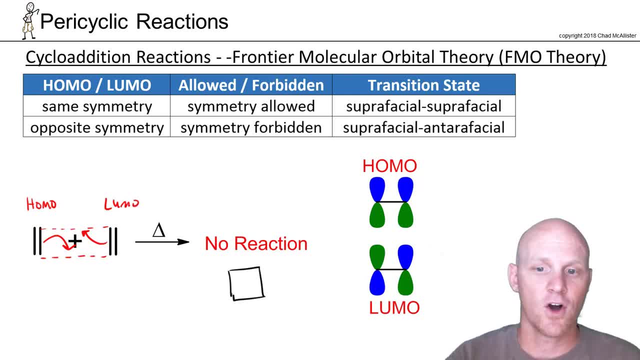 they're two identical reactants, so you just got to pick one. Well, in this case, we're going to. Well, in this case, the HOMO would be psi 1 and is going to be symmetric, whereas here the LUMO is going to be. 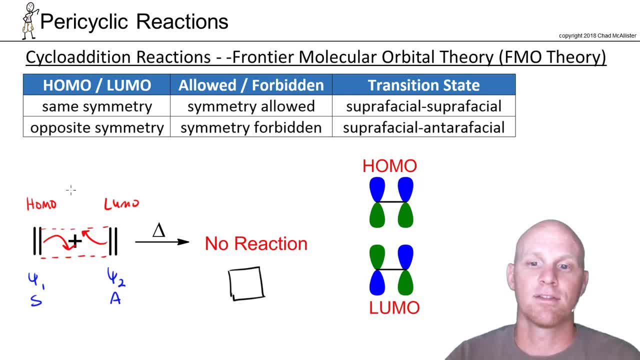 psi 2 and is going to be anti-symmetric and we can see that they have the opposite symmetry and therefore it is a symmetry forbidden reaction. So, and it's going to have to go by a superfacial and terafacial interaction if it's going to happen at all. Well, it turns out to have a. 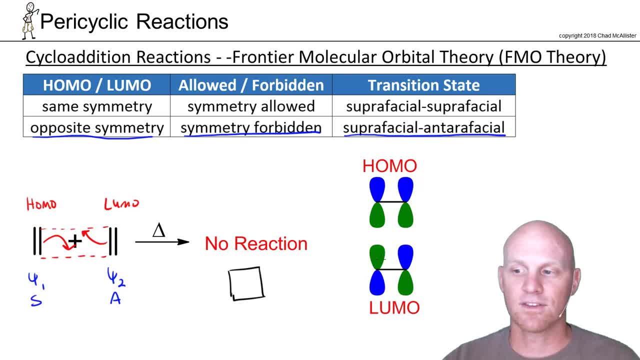 superfacial and terafacial arrangement here. If I need to, you know, kink one of these to make it happen. it turns out these both are too small for that to occur. So we also say that this is symmetrically forbidden. There's just not enough room to kink these enough to get that. 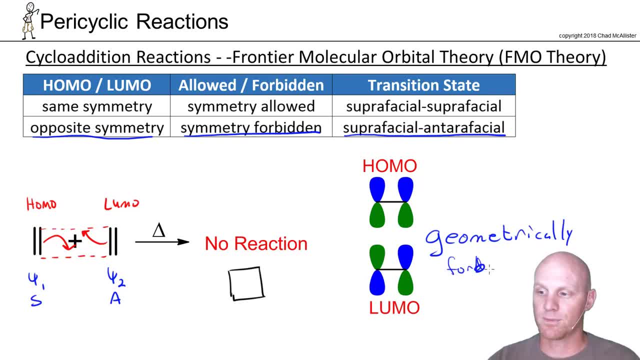 superfacial and terafacial interaction. I can spell forbidden putting Ds in the right places. So it turns out for just two ethylenes not going to happen. For the last example, as long as one of your reactants is more than two carbons, you can get it to happen. 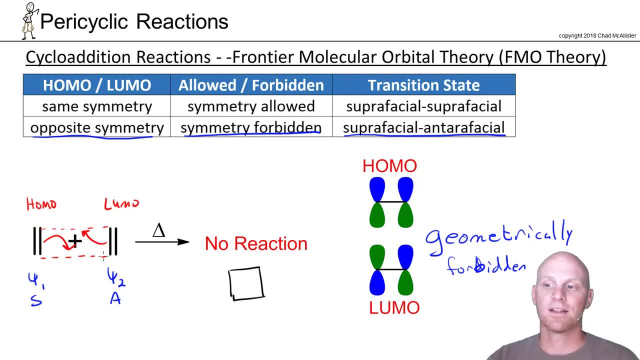 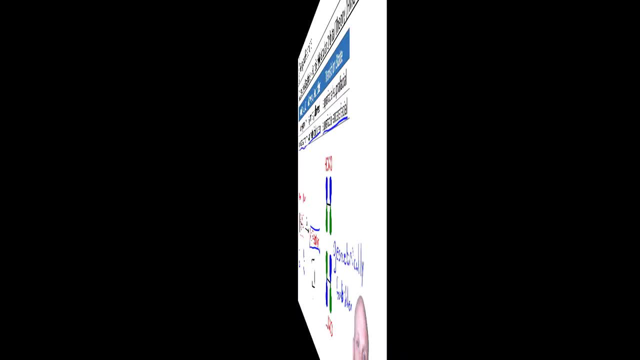 at least geometrically, even if it's symmetry forbidden. But for this one it's not just symmetry forbidden, it's also geometrically forbidden, and that's why we truly have no reaction here. So up until now, all the reactions we've been looking at have had this lovely triangle above. 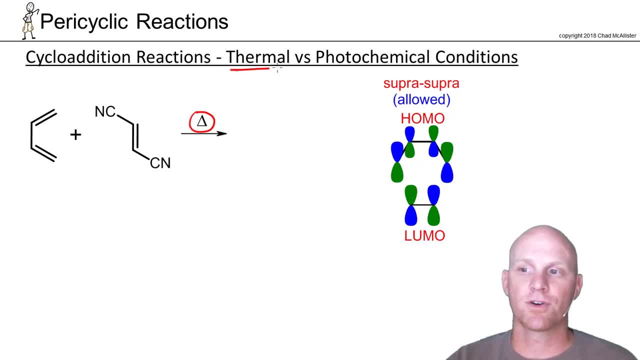 the arrow, and that just means heat, and we're going to call that thermal conditions. Well, it turns out, for most of your pericyclic reactions, you have thermal as well as photochemical conditions, And the big difference is that if you use light, using light of just the right energy- 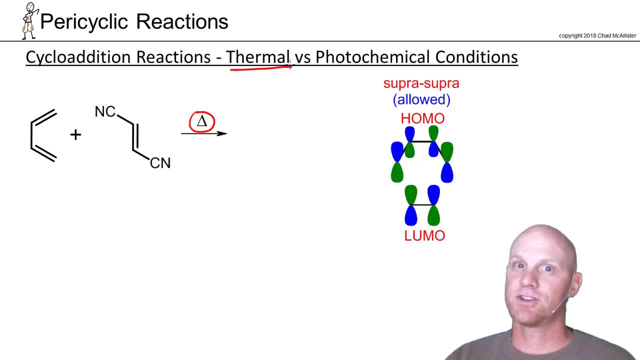 to promote electrons up to a higher energy orbital and it changes some things. So in this case I'm going to start with the Diels-Alder. We've looked at it pretty extensively and we kind of know how this goes In this case. 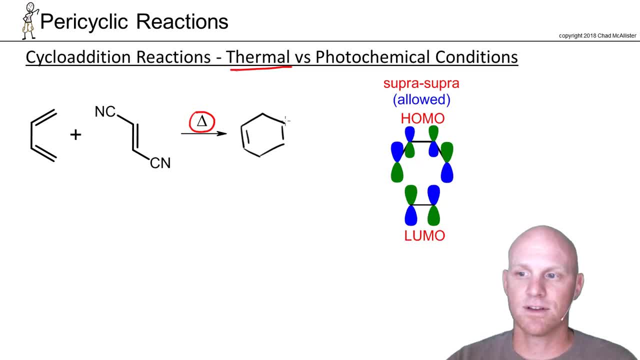 my product is going to look like this and I've got two cyanos that are trans to each other in the reactant, so they're going to be trans in the product. And so it turns out when you've got a reactant that's trans and then they're trans on the product, so in this case the dienophile's. 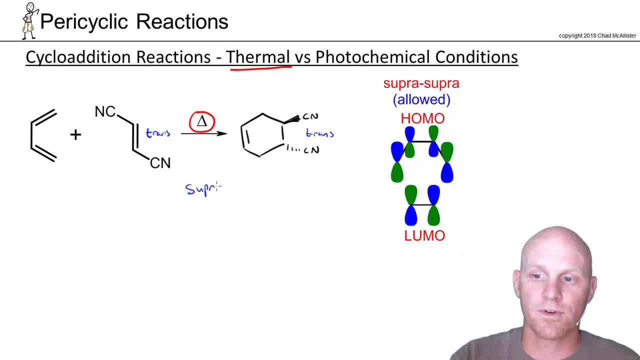 trans and then they're trans on the product. that's what suprafacial-suprafacial does. So when you have a suprafacial-suprafacial interactant, so a reaction I should say for a transition state: if your diene is trans, your product is trans. I should say sorry if your dienophile is trans. 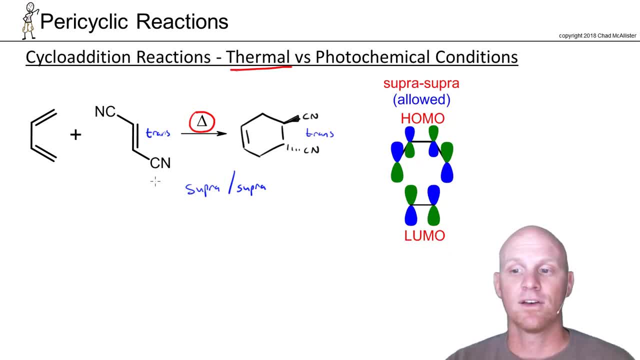 your product's going to be trans, and if your dienophile is cis, your product's going to be cis. So, however, if you have a supra-antera, suprafacial-anterafacial transition state, it would actually end up. 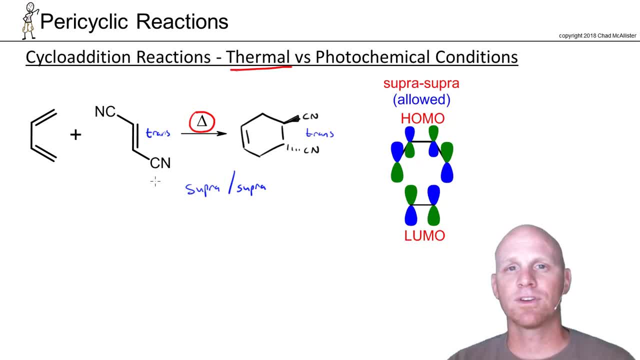 being the exact opposite situation. So you know what it looks like for Diels-Alder and I'm telling you, Diels-Alder is symmetry allowed and it's suprafacial-suprafacial. now you know kind of the stereochemical effects of suprafacial-suprafacial, Know that it's exactly the opposite for suprafacial-anterafacial. 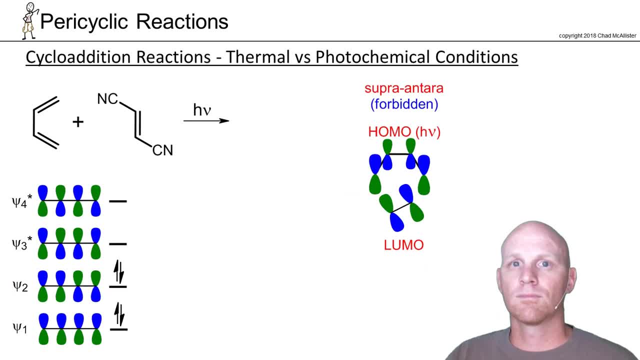 Let's take a look. Okay, so for the first time now over the arrow here, instead of heat we've got h? nu, and that's the energy of a photon of light. That's just our way of saying. we're using light and this is now photochemical conditions And this is. 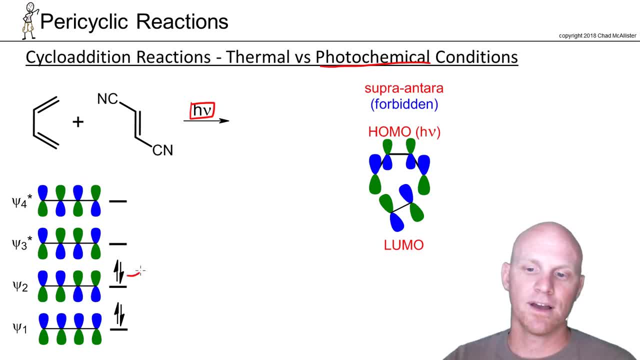 going to change some things. What the light does is it's going to promote electrons from psi 2 to psi 3.. So if you notice, normally this is the homo and that's the orbital involved in the reaction. But if all of a sudden I promote an, 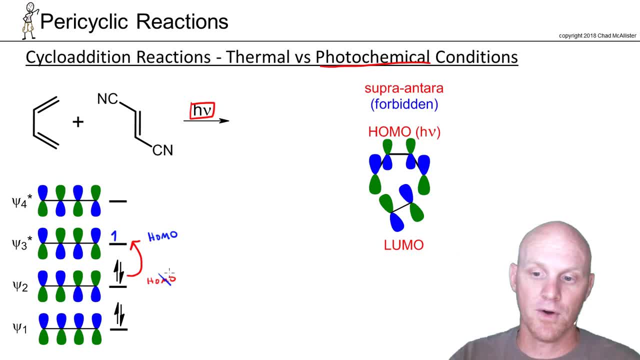 electron up here. this will now be the new homo, so, and this will now be the orbital involved in the interaction. And so notice, whereas psi 2 is anti-symmetric, we can see that psi 3 is symmetric. And so here this lovely symmetric orbital. 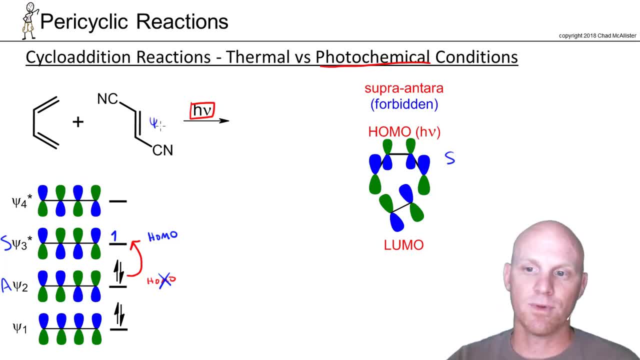 interacting with ethylene. well again, ethylene's LUMO is psi 2, which is anti-symmetric, And so I've got a symmetric trying to interact with an anti-symmetric, and that is symmetry forbidden. So, and if you recall symmetry, 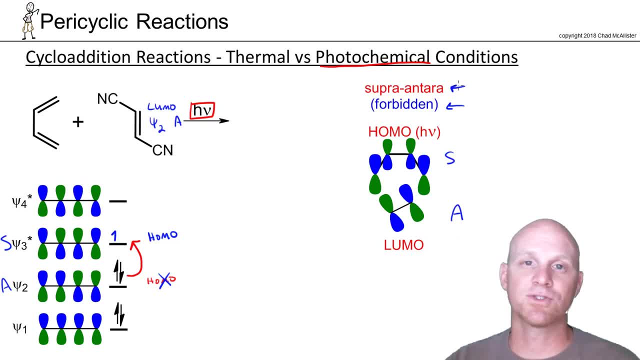 forbidden implies a suprafacial and terafacial transition state, And so, in this case, we should know that what we might expect is exactly the opposite of what we normally saw in a Diels-Alder, which is suprafacial, suprafacial. So here the two. 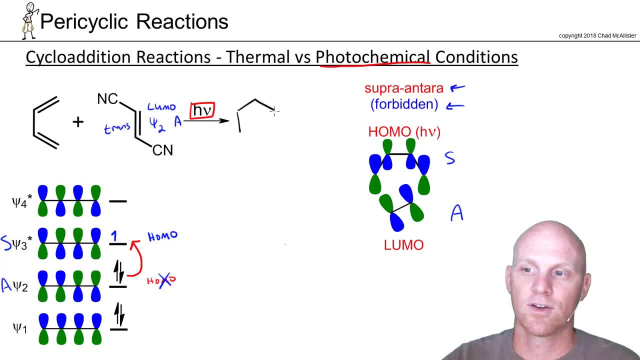 cyanide groups are trans to each other, but in the product they now have a chance of ending up cis, And this is a meso compound, so you don't got to draw both versions, And so stereochemically we also see a difference between 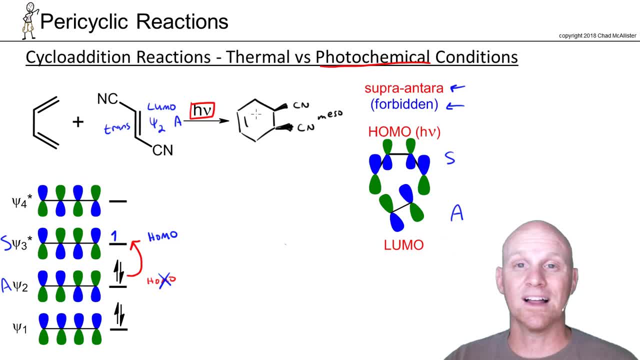 thermal and photochemical conditions. So, whether you do a symmetry allowed, reaction suprafacial, suprafacial- or a symmetry forbidden, reaction suprafacial and terafacial.